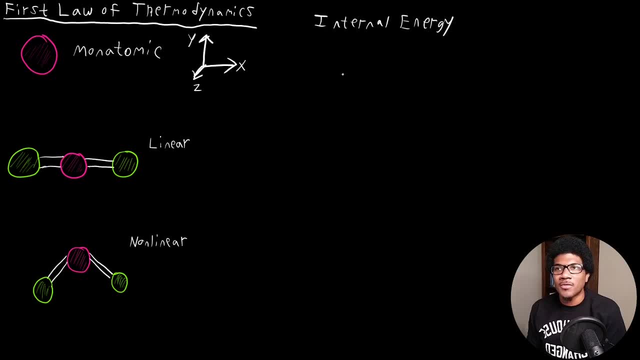 can happen to molecules, right? So it's associated with the motion of molecules And we use the letter U, so a capital U, to denote internal energy. Now, as far as this calculation, you're more or less familiar with this idea of energy being a sum of kinetic and potential contributions. 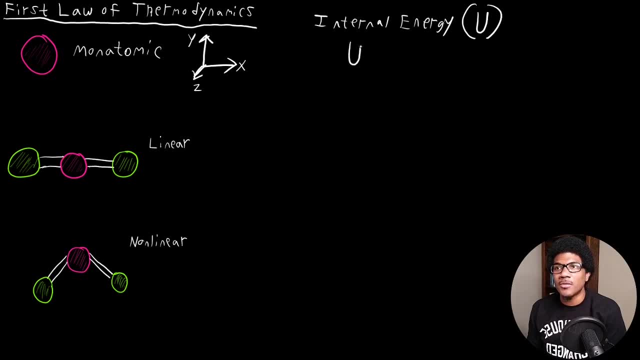 And that's exactly what the internal energy is as well. So the internal energy is just a sum of the kinetic energy and the potential energy. So I'll denote kinetic energy as Ke and potential energy as Pe, And internal energy is just a sum of the kinetic energy and 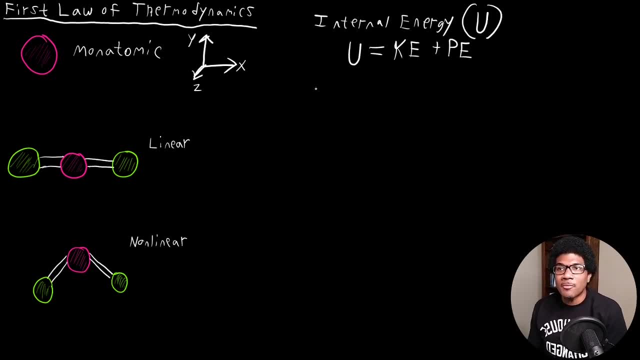 of both of those components. Now, if we assume an ideal gas, remember that one of the assumptions of the ideal gas law is that the molecules don't interact with one another. right, We're assuming they're just billiard balls. they bounce around and they hit each other, but there's no energy. 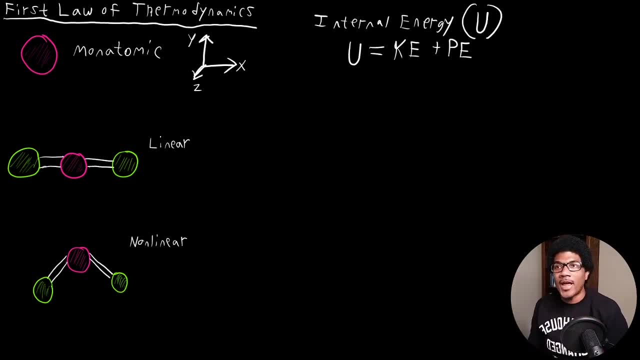 between them, There's no potential energy of their interaction. So what that means is that for an ideal gas, right PE is going to be equal to zero right. So for an ideal gas, this potential energy is going to be equal to zero. So the internal energy is only going to depend on the kinetic. 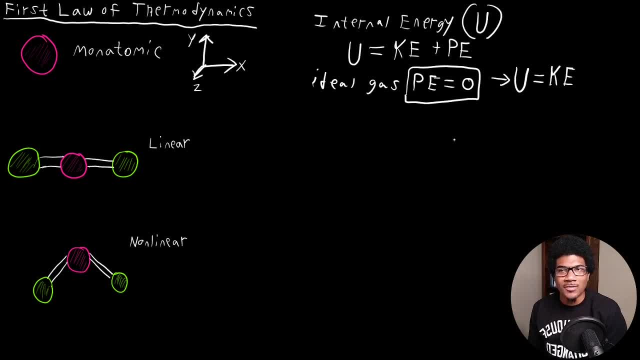 energy contribution. So this simplifies our equations greatly right, And it simplifies our discussion of internal energy. Now, in one of the very first videos, I mentioned something called the equipartition theorem from statistical mechanics, and it introduced something called the degrees of freedom that are available. 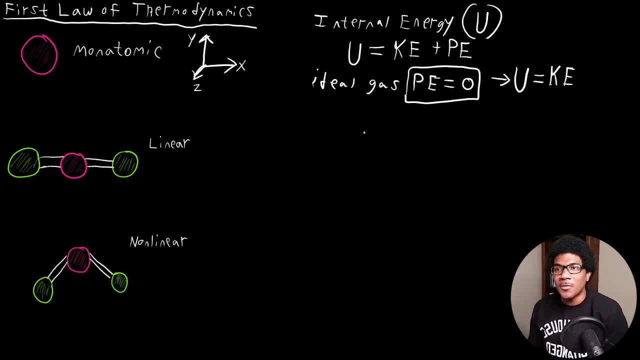 to a molecule or to a particle right. So we basically define the internal energy using this, these degrees of freedom. So U is going to be equal to the degrees of freedom divided by two times NRT. Now, youivendoque heb Universi d' Hebrews, okay. 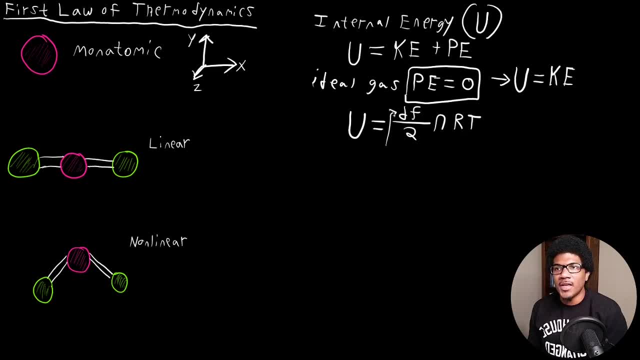 right. so this df is the degrees of freedom, And this is going to depend on the identity of your gas particles, particularly their molecular shape. But this is more or less the equation for internal energy. U is going to be equal to the degrees of freedom over two, Now the degrees. 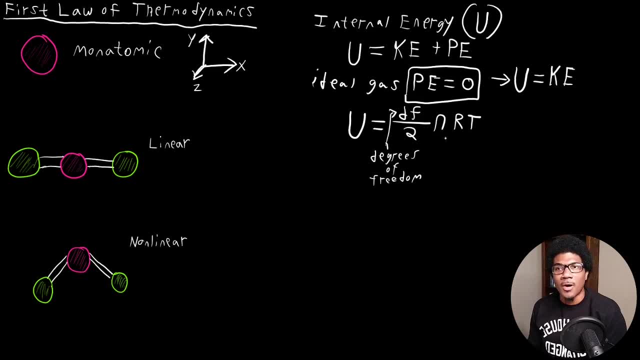 of freedom in this case are either going to be associated with delta or somewhere else. And in the real energy equation, I'm going to use delta or � as an example. We'll talk about that after this. to be associated with translational motion or rotational motion now for a 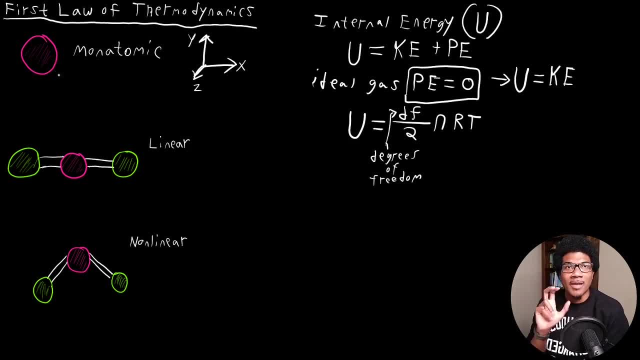 monatomic gas. think about this: if you rotate a monatomic, just a single atom, right, if this, if we're approximating it as a sphere, it's going to be spherically symmetric all the way around. so if you rotate it, there's no change in its. 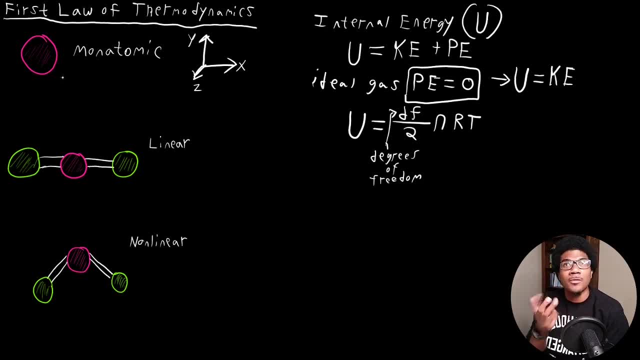 representation: right. so you rotate an atom, it's spherically symmetric. so it doesn't matter where you rotate it or which axis you rotate it around, it's going to have the same representation. so that means that a monatomic gas will only have three degrees of freedom. right? so for a monatomic gas, DF would be equal. 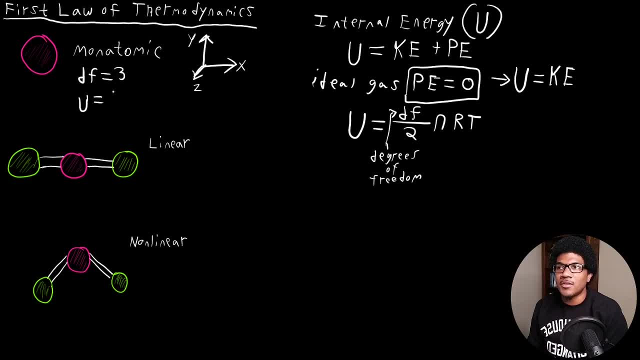 to three, and so that means that your internal energy is going to be three halves in RT. right, so this would be your internal energy for a monatomic gas, because it only has three degrees of freedom, the three degrees associated with its translational motion. now, as we start to look at more complicated molecules, they begin to have 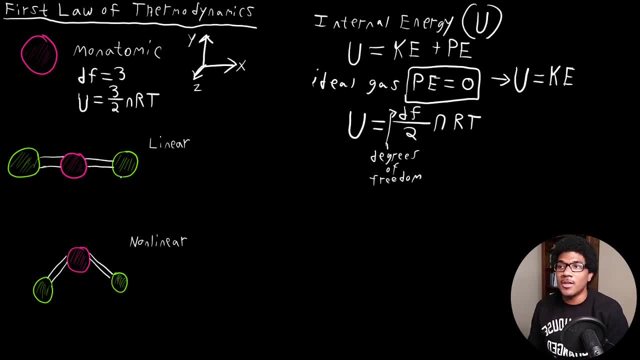 more degrees of freedom. so let's take the case of a linear molecule and let's note our axis system. so the horizontal axis is X, verticals Y, and coming in and out of the board is going to be Z. so I guess coming in, out of the screen for 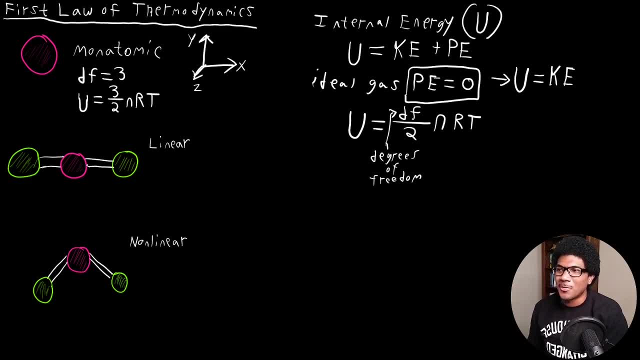 you guys perspective. so so for a linear molecule we're going to have two additional degrees of freedom if you rotate it around the visible axis, let's say around the Y axis. so let's say you define this axis and you pull a rotation around that axis. right, that's going to give you a unique representation. 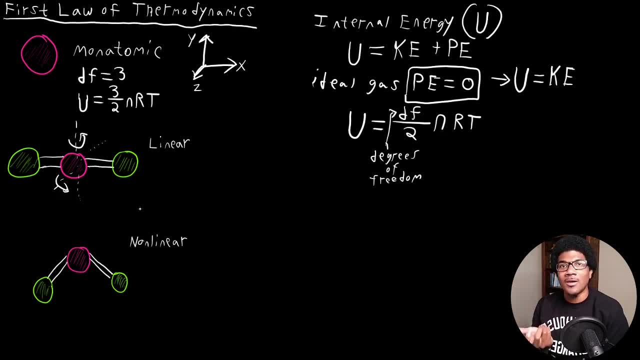 for each time you rotate it. also if you rotate it around the z-axis. so this is the access coming in and out of the screen. you rotate around that axis for each time you rotate it into the Y axis. if you rotate it around the X located into the facing of it in order for it to rotate. and that finalized it back to board in order for near Antonio is random, her pivoting around the partial growth. but if the wall is ever in alignment to the Daddy tire rotation, that promote you a unique representation of the molecule rotating it around theложal area is going to give you a unique representation of the molecule rotating it around the axis. word-by-word: co-ire-s ordinance, сос-ah-standarden- jig-sar-s: how to interpretation★. 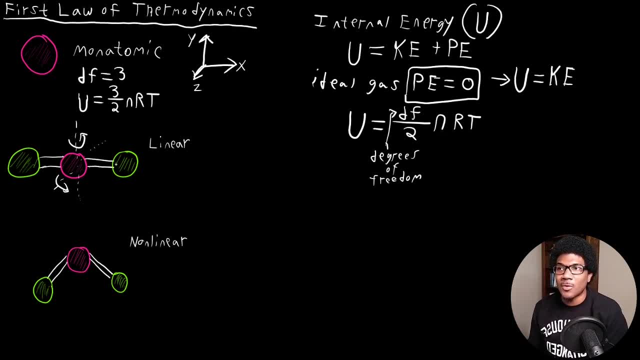 However, you do not get a unique representation rotating around the x-axis right, Because you're just rotating it. It's kind of similar to when you rotate the atom. You don't really change the molecule's representation by rotating it that way. 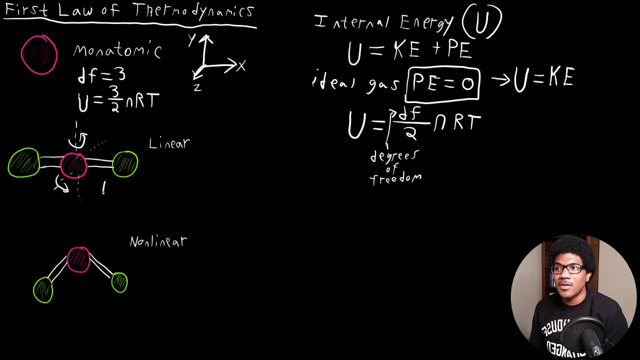 So you end up with two additional degrees of freedom. So in this case, for a linear gas, the degrees of freedom would be 5.. So that would give you the internal energy expression of 5 halves nRT. OK, so now for a nonlinear gas, you have the three translational degrees of freedom. 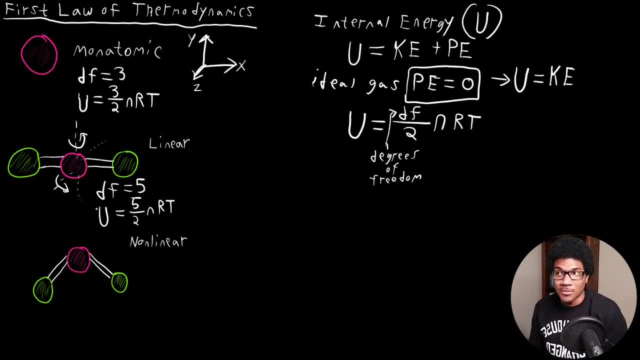 You have those two rotational degrees of freedom around the y and the z-axis, But you also have an additional rotational degree of freedom around the x-axis as well. right, If you rotate around that axis, you also change the representation of the molecule. 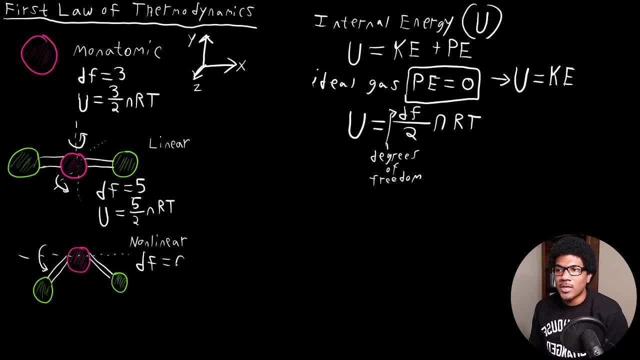 So in this case, dx And f is going to be equal to 6,, right? You're going to have 6 total degrees of freedom, And for the internal energy for this guy that would just be 3 nRT, right. 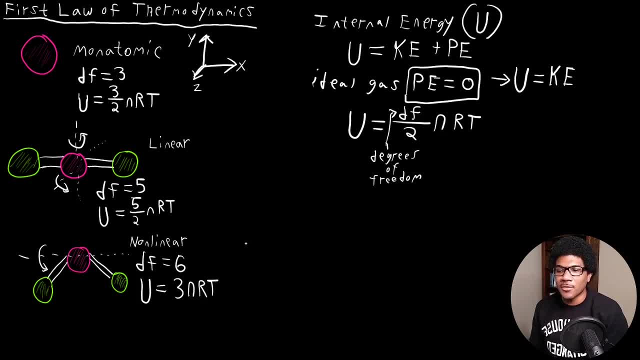 So these are going to be your differing internal energy expressions, based on whether your gas is monatomic, linear or nonlinear. Now, the first law of thermodynamics deals with this concept of internal energy And basically it says that energy cannot be created nor destroyed, right? 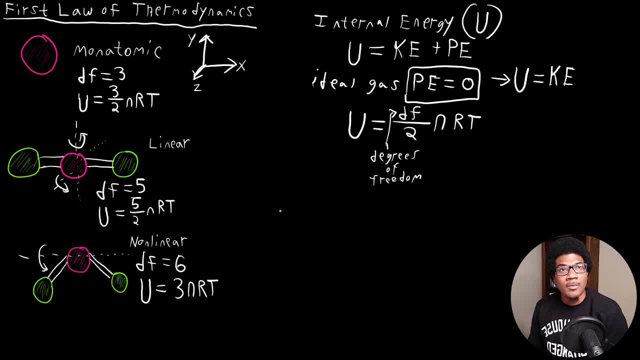 So that's the statement of the first law of thermodynamics. So inherently it deals with an energy change right. It's basically saying that your delta U right is going to be. it can't be created nor destroyed. It has to be transferred, right. 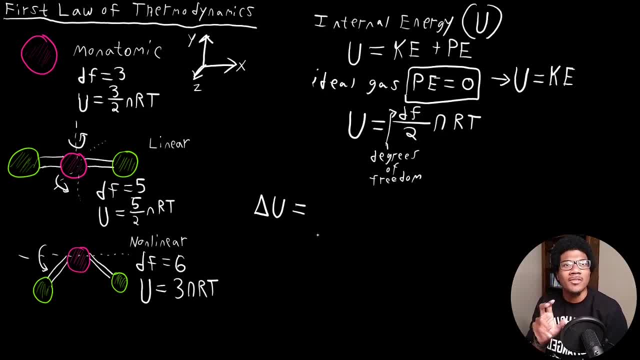 So that's kind of what I always like, to add that to the first law of thermodynamics statement: Energy can't be created nor destroyed. It can only be transferred. And it can be transferred through two mechanisms. One is heat, which we use the lowercase q to define heat. 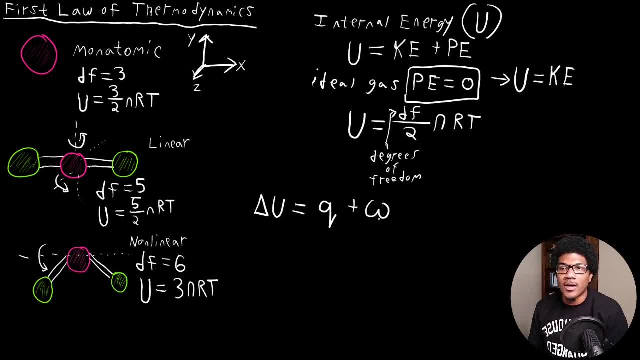 And work, which I use, the lowercase w Kind of looks like an omega. Let me do w there right. So q plus w, So you can only transfer energy in the form of heat and work. So that's the whole statement of the first law of thermodynamics. 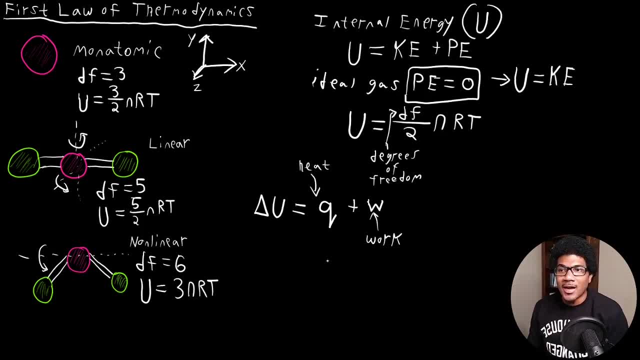 Energy cannot be created nor destroyed. It can only be transferred. Okay, And this will lead to a differential expression as well, So you could also have: du is equal to dq plus dw, right? So you can also have a differential version of that expression. 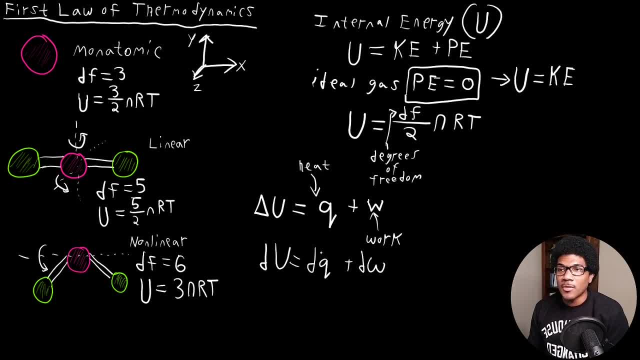 As well, right, So yeah, so this is a statement of the first law, Mathematical statement of the first law of thermodynamics. Now I do want to talk a little bit about the sign conventions for q and w, for heat and work. 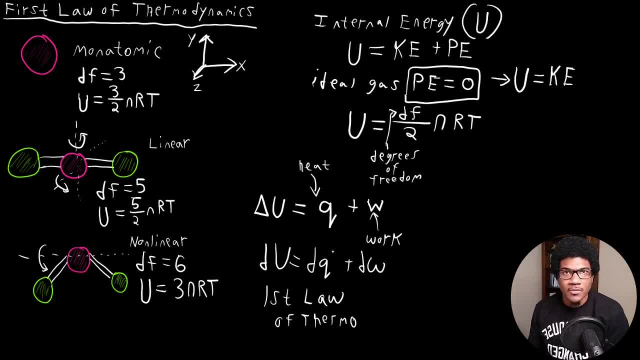 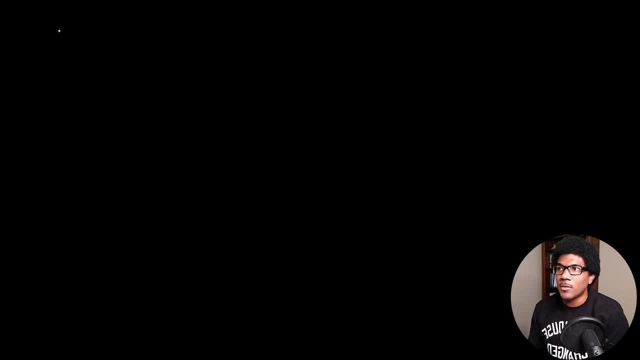 So these can be positive or negative numbers And they're going to mean something different in both cases, right? So let me go to a new slide here. So let's say, for example, we have a positive q, Right? So if we have a positive q, that means that the system is gaining heat, right? 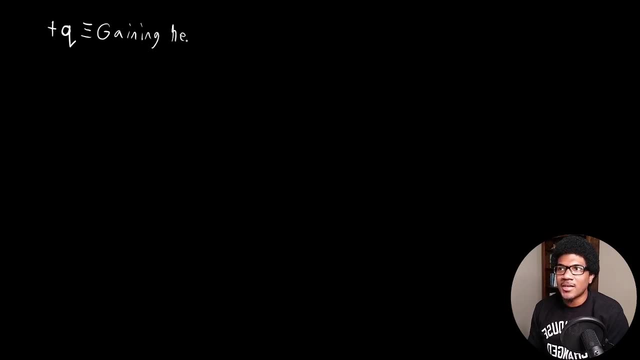 So positive q, we are gaining heat. For a negative q, that means that the system is losing heat, Right? And so this always depends on what you define as the system, right? So, kind of going back to our- you know- original video on defining thermodynamic systems, whatever, 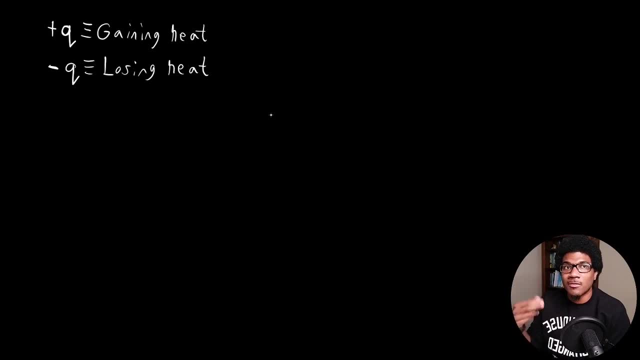 you define as the system is going to influence the signs of these of heat, and work right. If the system is gaining heat, you'll end up with a positive q, And if it's negative q, that means that the system is gaining heat. 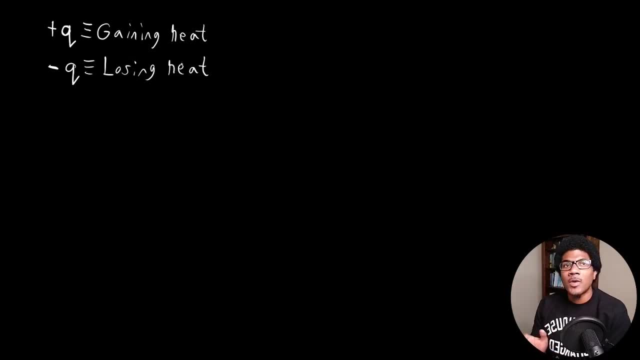 That means that the system is losing heat, And a good way to think about this is to kind of think about these as total changes. right, If your system is gaining heat, then you know the total change is going to be, you know. 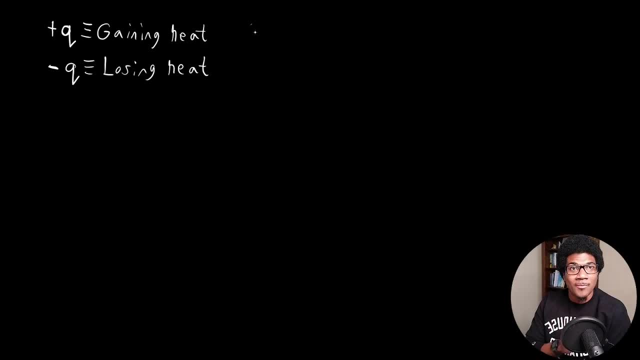 the total change of some variable is final minus initial. If you're gaining heat, that means your- you know- final heat value would be greater than your initial heat value. So that means there will be a positive number. Same thing with losing heat.